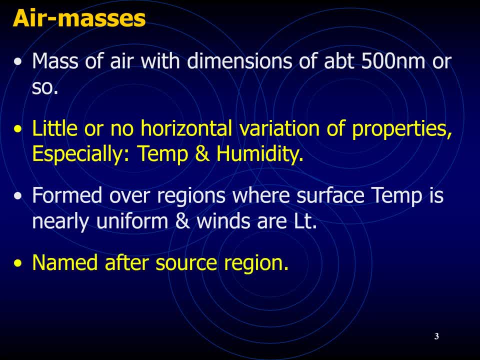 When a geographical position lies within an air mass of particular type, the weather experienced will be characteristic of that air mass. They are named or they originate from what we known as source regions. In order for a huge mass of air to develop uniformly, same characteristics is source region should be. 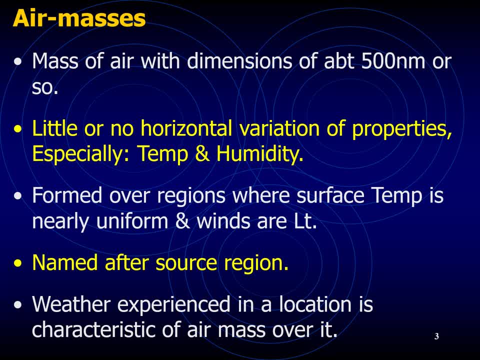 defined as the air mass of a flat and of uniform composition with light surface winds. The longer the air remains stagnant over its source region or the longer the path over which the air moves, the more likely it will acquire properties of the surface below. Consequently, ideal source regions are usually 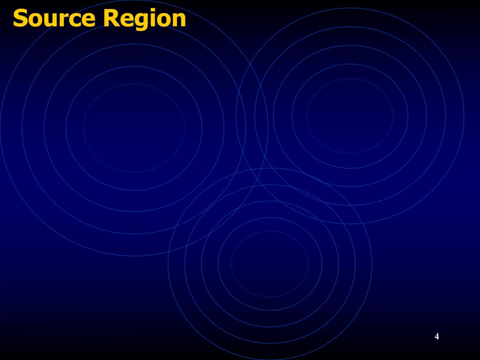 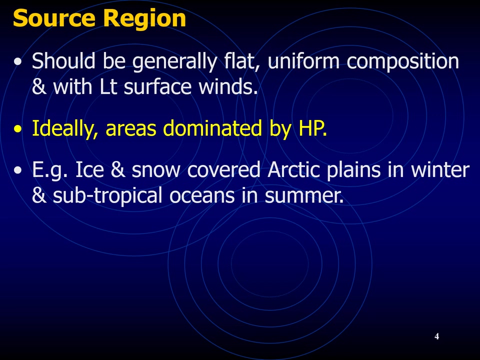 those areas dominated by surface high pressure. They include the ice and snow-covered Arctic plains in winter and subtropical oceans in summer. The middle latitudes, where surface temperatures and moisture characteristics vary considerably, are not good source regions. Instead, this region is a transition zone where air masses with different physical properties move in, clash and produce an exciting array of weather activity. 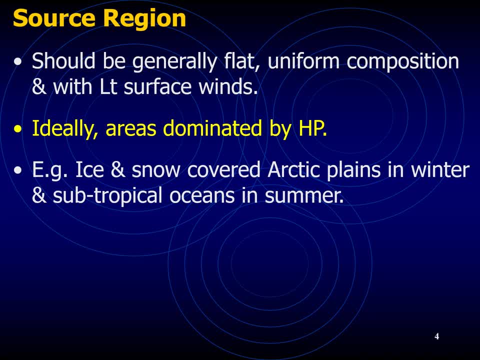 Factors that affect the properties of an air mass, like the temperature and soil temperature, may also be Typically high by temperature. We can also find the direct factors of positive air mass, like the air atmosphere temperature and temperature of the air. However, to be completely clear, the image of the area of the air mass is not consistent with the area of the air mass. 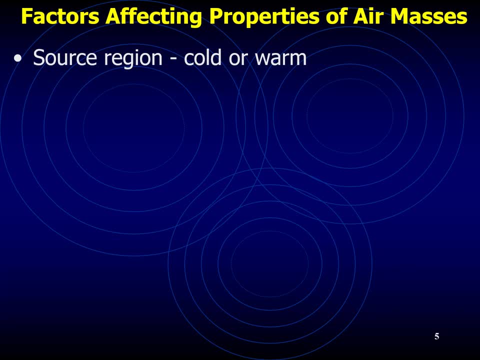 To be completely clear, the image of the area of the air mass is not consistent with the area of the air mass, As a high energy source will provide a wave of electric current. Instead, such energy will produce a wave of electric current. 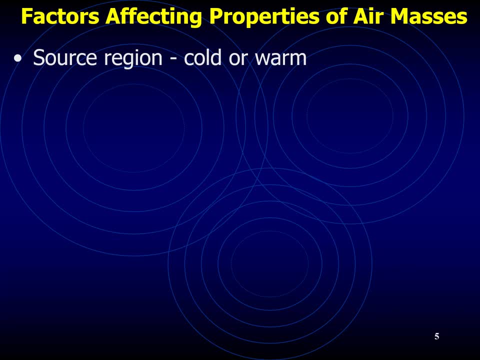 Now, how does the air mass affect the air mass, like I talked about already, source region where the temperature would depend on whether it is of polar origin or tropical origin. The track over the earth's surface, that is, the terrain, will determine if it will be a dry air mass or a moist air mass. Extent of convergence or divergence. 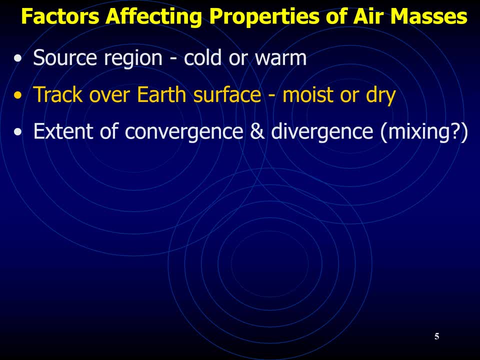 which results in mixing of air, thus influencing the properties such as relative humidity and lapse rate. Number of days spent in source region, that is, the age of the air mass Properties would depend on the time that has elapsed since it left the source region And, finally, the rate of travel. 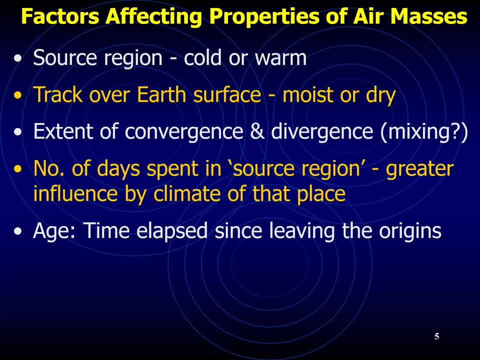 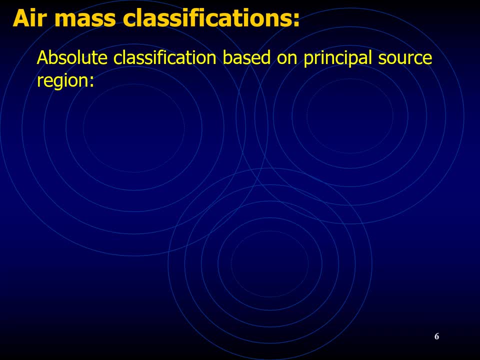 how long the air mass will retain its original properties would depend on the time spent on a particular region outside its source region. Air mass classification is as follows: An absolute classification is a classification of the air mass of a particular region outside its source region. 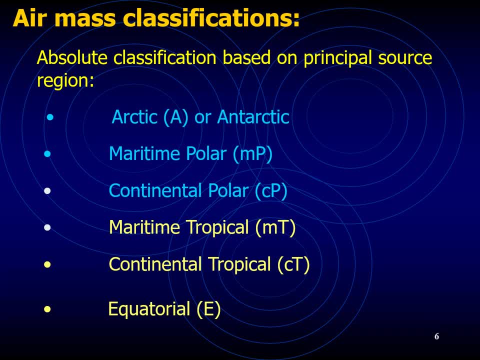 The classification based on the principal source region of air masses is as follows. For example, a continental polar and continental arctic air masses are those air masses which comprises of the bitterly cold weather that invades southern Canada and the United States in winter and associated with continental polar and continental arctic air masses. These air masses originate over the ice and snow covered regions of the earth. 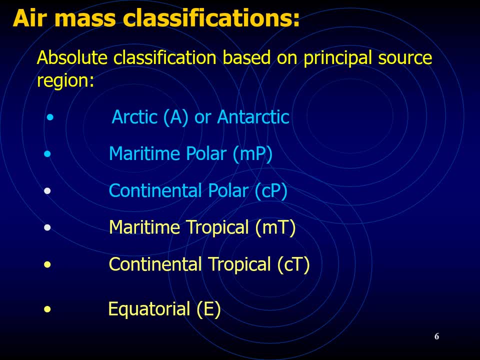 Northern Canada and Alaska, where long clear nights allow for strong radiation cooling of the surface. Air in contact with the surface becomes quite cold and stable, since lethal moisture is added to the air. it is also quite dry and specific humidities are often less than 0.3 grams per kilogram. Another example are the maritime polar air masses Now during the winter. 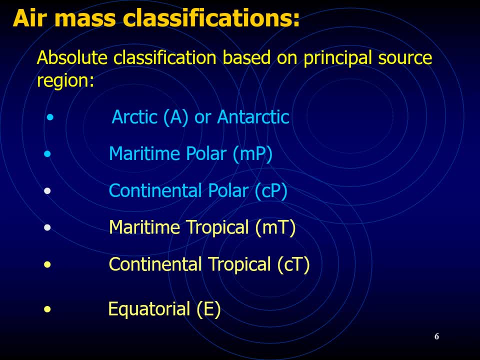 continental polar and continental air originating over Asia and frozen polar regions is carried eastward and southward over the Pacific Ocean by the circulation around the Aleutian low. The ocean water modifies these cold air masses by adding warmth and moisture to them. Since this 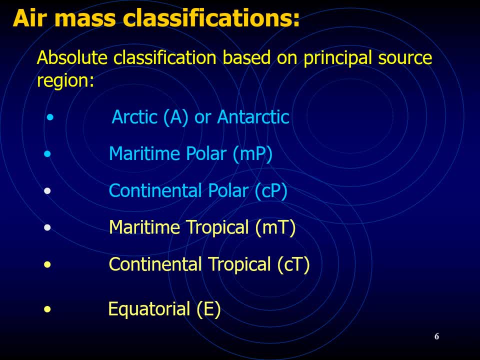 air travels across many hundreds of, even thousands, of kilometers of water. it gradually changes into maritime polar air. Now I can talk about all these air masses, but you get the idea right. So the wintertime source region for Pacific maritime tropical air masses is the subtropical. 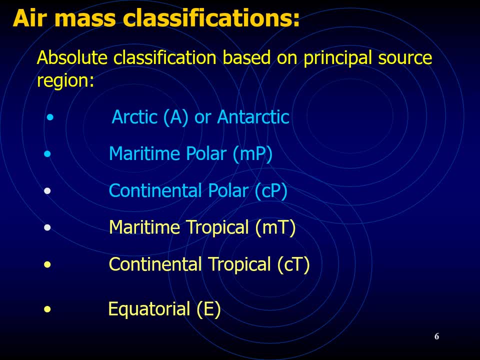 east Pacific Ocean. The only real source region for hot, dry continental tropic air masses in North America is found during the summer in northern Mexico and the adjacent arid southwest United States. Here the air mass is hot, dry and condensate. The air mass is hot, dry and condensate. Here the air mass is hot, dry and condensate. Here the air mass is hot, dry and condensate. The air mass is hot, dry and condensate. Here the air mass is hot, dry and condensate. 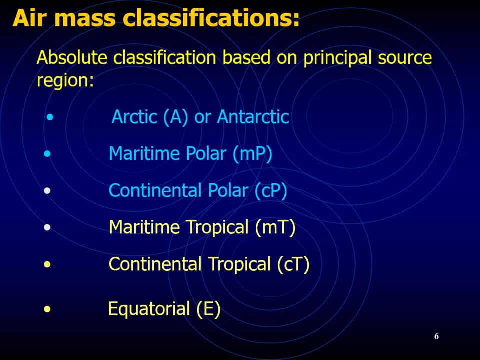 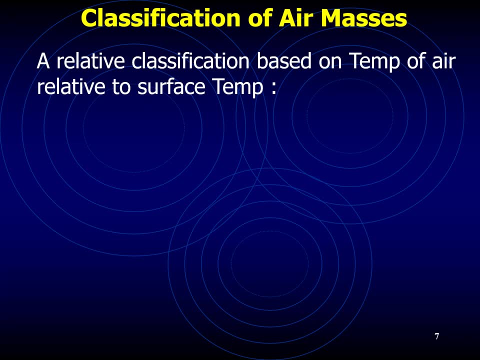 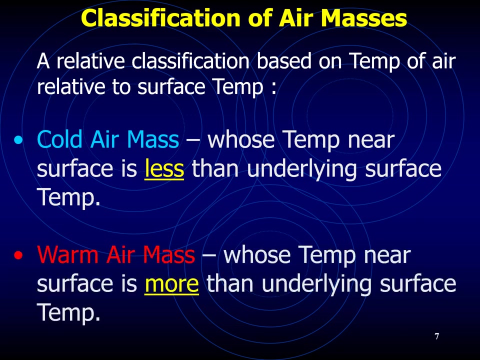 Unstable at low levels, with frequent dust devils formed during the day. Classification of the air masses based on the temperature of the air relative to the land or sea surface temperature are cold air mass, whose temperature near the surface is below the temperature of the underlying surface and warm air mass, whose temperature near the surface is. 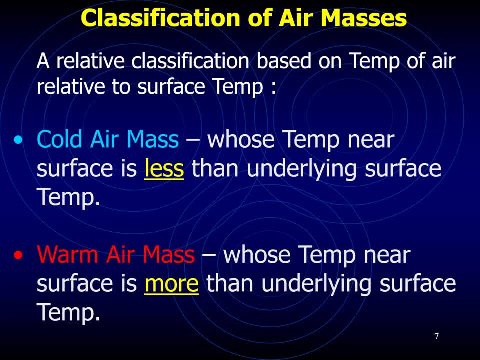 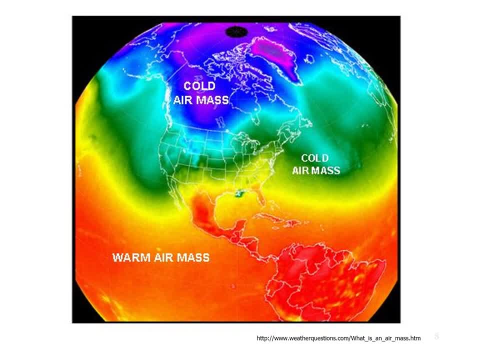 above the temperature of the underlying surface. Here you can see a thermal diagram of the cold air mass and the warm air mass is shown, where temperatures- the brighter the color, the higher is the temperature of the air mass. Cold air is being warmed from beneath and tends to be thermally unstable with cumulus. 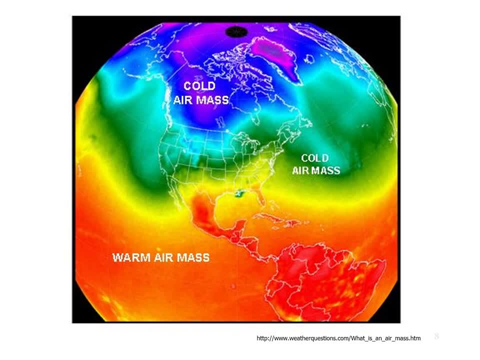 type clouds and good visibility, except in showers. Warm air is being cooled from beneath and tends to be thermally stable, with stratified cloud and possibly fog. As long as there is no fundamental change in the type of air mass, there is not likely to be any important changes in the weather. 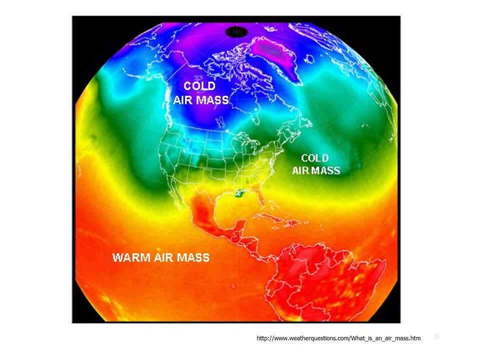 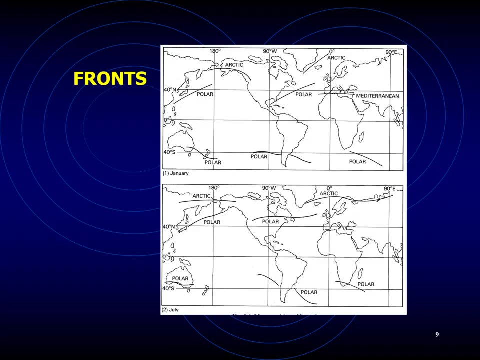 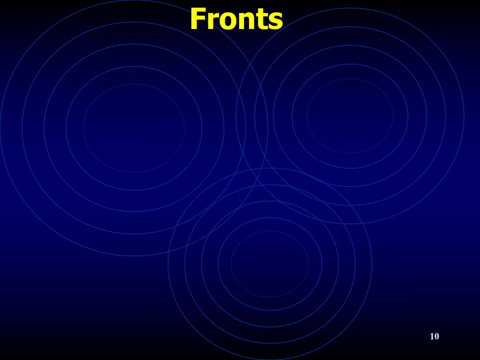 However, when the air mass changes in their property, so too will the characteristics of the weather. So an interaction of air masses leads to the formation of a front, and you can see the location of the fronts based on their geographic location. Now lets talk about the warm front and the cold front. 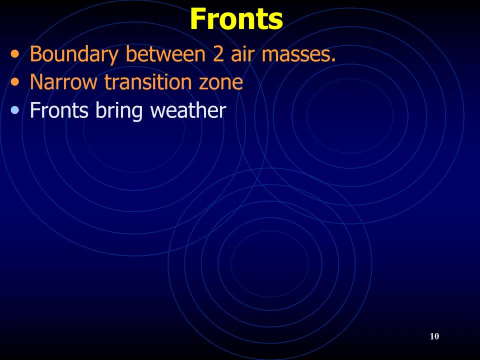 Now, a front is the transition zone between two air masses of different densities. Since density differences are most often caused by temperature differences, fronts usually separate air masses with contrasting temperatures. Often they separate air masses with different humidities as well. Remember that air masses have both horizontal and vertical extent. 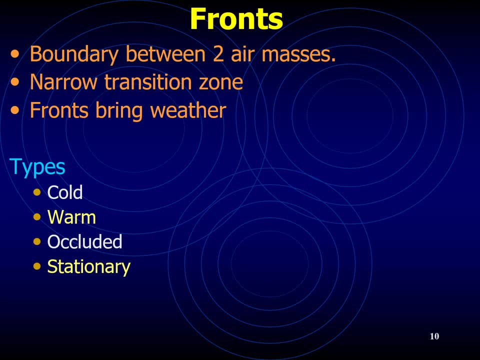 Consequently, the upward extension of a front is referred to as a frontal surface or a frontal zone. Now there are four types of fronts: cold fronts, warm fronts, occluded fronts and stationary fronts. At a cold front, cold air replaces warm air at a given place. 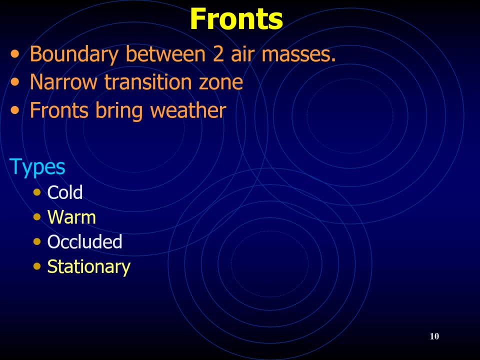 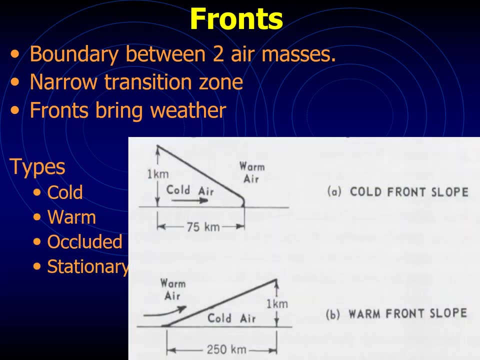 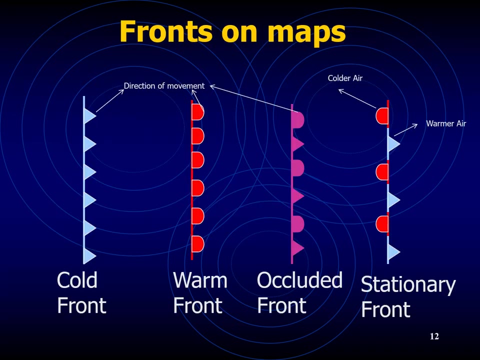 At a warm front, warm air replaces cold. In both cases, warm air rises above the cold front. In both cases, warm air rises above the cold front. In both cases, warm air rises above the cold front. That is how Erdeong passes above the cold air at the front. 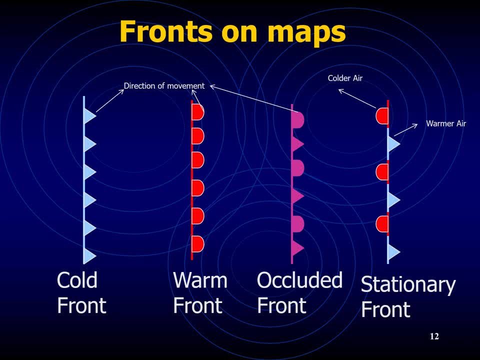 A stationary front has essentially no movement. garment movement. on a colored weather sheet, A stationary front is drawn as an alternating red and blue line. Semi circles face towards colder air on the red line and triangles point towards warmer air on the blue line. Theses forces quickly change on both occasions. 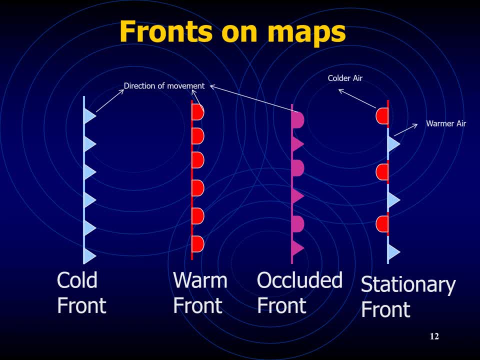 Depressions often originate in the flow, about 2 to 3 m units. It is safe to assume that last few years there sometimes are less feeds but not enough when on a front such as at the stationary front that exists between polar and tropical air masses, also called the polar front here polar easterlies and 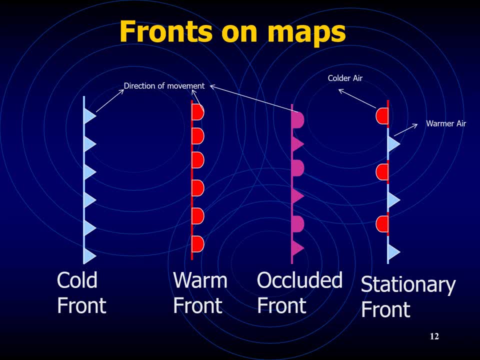 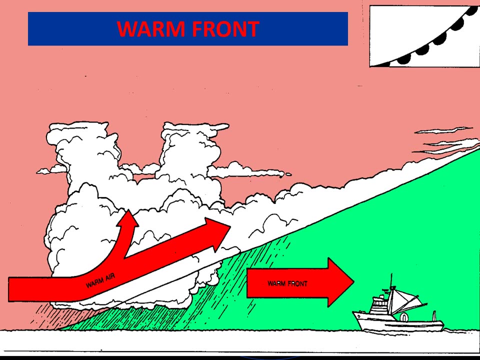 temperate westerlies are in close proximity. in general, a depression starts as a small wave like disturbance on a frontal surface. the bulge of the wave is towards the cold air. some of these waves undergo little or no change and eventually die down. some waves, however, increase in amplitude as the bulge 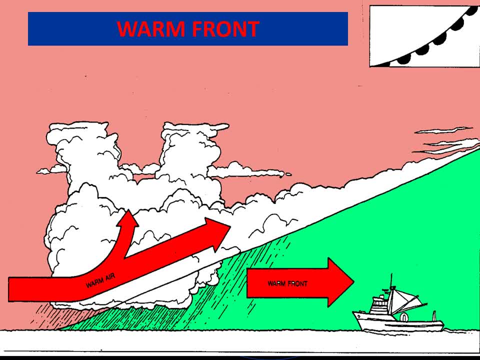 becomes larger, pressure begins to fall, with the largest fall at the tip. therefore, a closed system of isobars develop. as the depression develops, it also starts moving generally in the same direction as that of the warm air. now we've covered depression in my previous video, when we talked about me latitude. 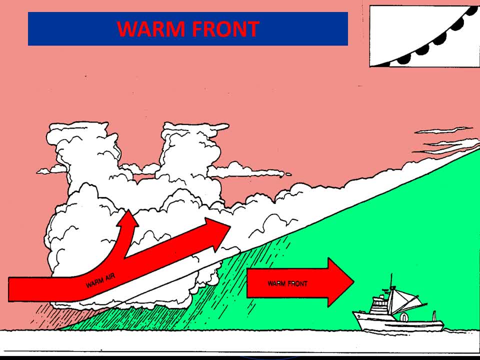 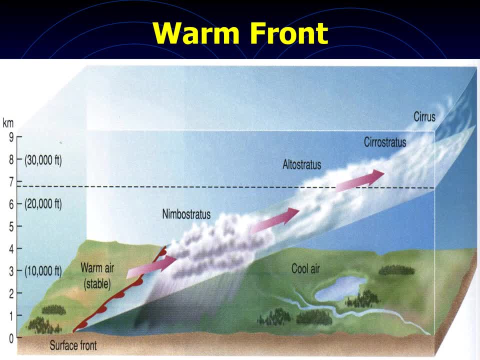 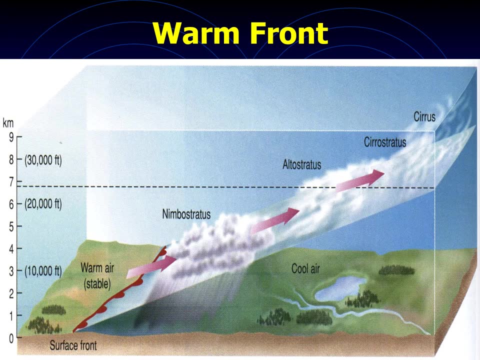 depressions and extra tropical cyclones, so I will not go too deep into that you. what I will discuss here is the weather on passage of a warm front. so warm fronts have a lesser slope, so the passage of the front takes longer and the weather changes are therefore more spread out and less violent than at a 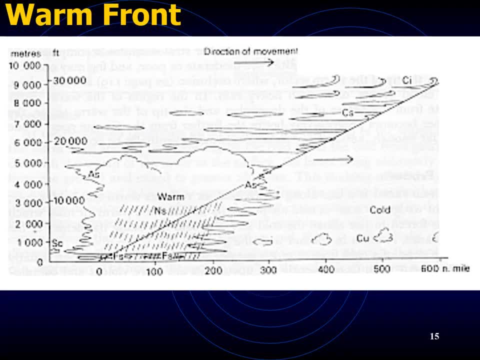 cold front. if you approach a warm front, the pressure will steadily fall in advance. steady pressure will be there during the passage and changing to slow fall after the passage. the wind will shift to southwesterly or South in the northern hemisphere and northwesterly or in Southern Hemisphere and freshening later, wearing in the. 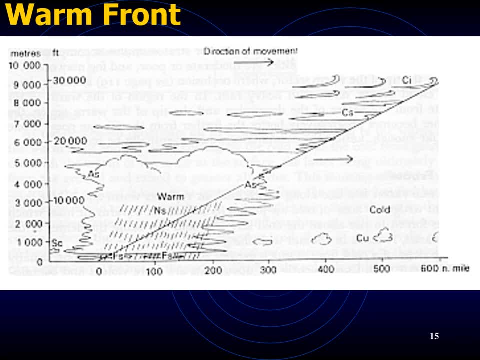 North Hemisphere and backing in the Southern Hemisphere can be observed. temperature will steadily rise as you approach the warm front. in terms of clouds, initially the cedars, pumulus and altostratus and nimbostratus in succession in advance are formed. then lower nimbostratus are formed in succession in advance, then lower nimbostratus in succession. if the 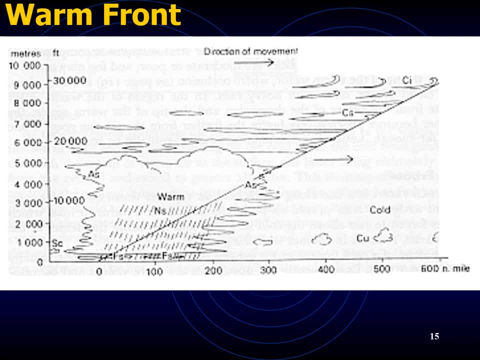 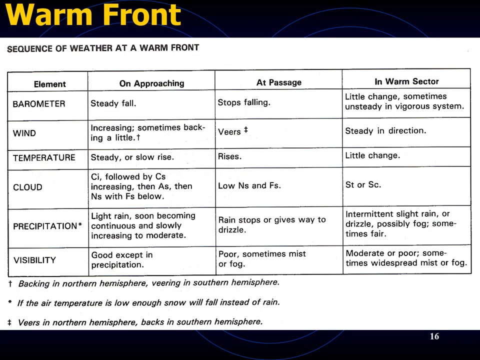 has passage and stratus or stratocumulus is formed at the rear of the warm front. In terms of weather, we have continuous rain or snow before the front, stopping or turning to drizzle after passage. The visibility is generally good, except in rain ahead of the front becoming poor during and after passage. We now will. 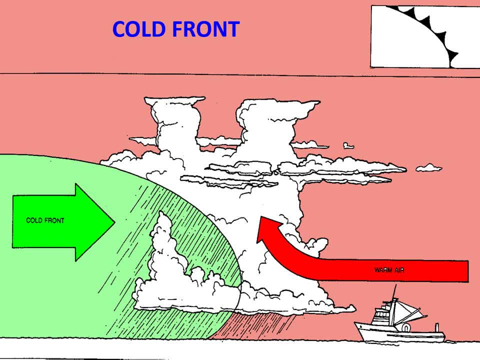 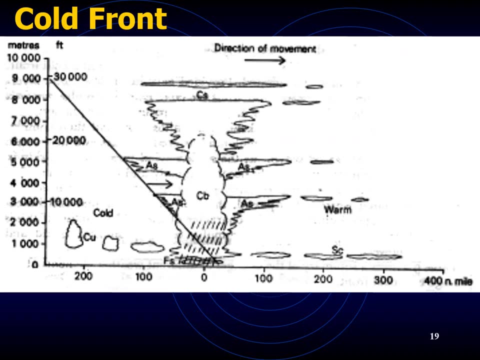 discuss the weather on passage of a cold front. Cold fronts generally slop comparatively steeply and produce active cloud and showery precipitation and sometimes even thunderstorms, Continous coldicipations. The weather associated with the cold front is as follows: The pressure starts to fall as you approach a cold front, with a sudden rise. 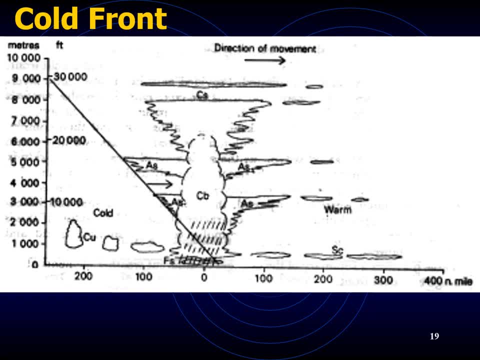 at the front, then a slow rise at the rear. In terms of the wind, you observe varying topical astonishing pressure. Several smallstonings are also present, but of course there should be a steady rise or reddish rise, as the front时 an energy. 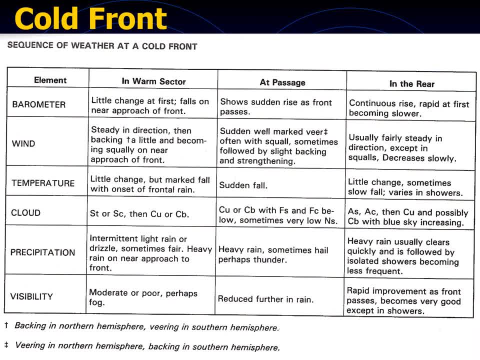 the west or northwest in the northern hemisphere and backing the west or southwest in the southern hemisphere, often squally. the temperature suddenly falls as the front passes. in terms of clouds, we start with the autocumulus or autostratus, then heavy cumulonimbus in advance and passage. 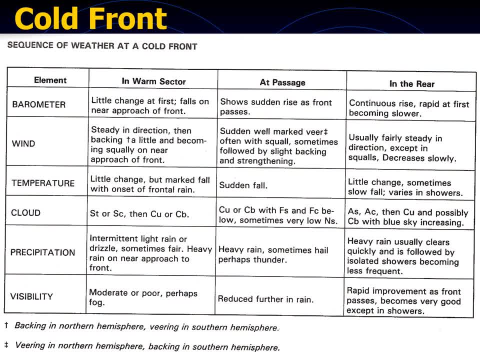 cloud base lifts rapidly after passage, followed by autostratus or autocumulus, and later cumulus or cumulonimbus. in terms of weather, we experience rain, perhaps even thunder, which increases during passage and then turns to showers. the difference between precipitation in the cold front and a 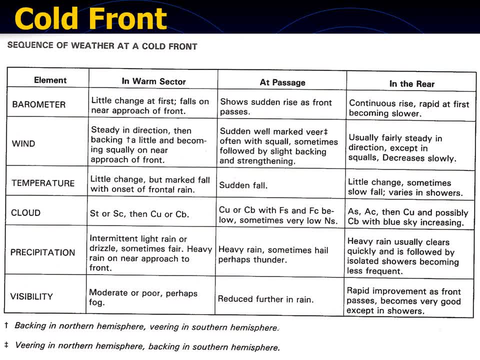 warm front is that precipitation in a cold front is more intense. it may last shorter in comparison, but it is more intense and heavy and severely affects the visibility. whereas the precipitation during a warm front is light and steady, but it goes on for a longer time, a visibility during the cold front or passing of a cold front is generally poor.